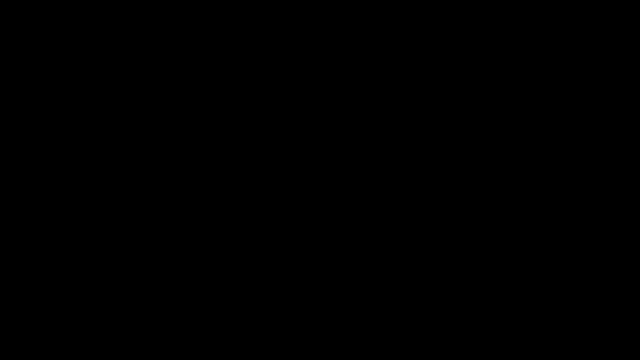 In this video we're going to focus on multiplying numbers with decimals. So let's start with a basic example. first, What is 4.6 multiplied by 7?? Well, first we need to multiply 6 times 7.. 6 times 7 is 42. So we need to put the first number, 2, and carry over the 4.. Next, let's multiply 4 times 7.. 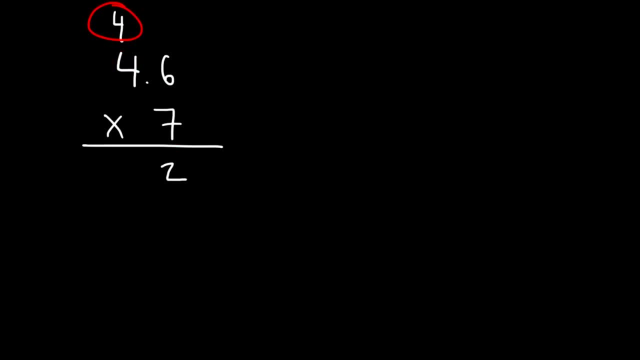 4 times 7 is 28 and we need to add the 4 on top. 28 plus 4, that's 32.. Now notice that we have one number to the right of a decimal point. So therefore in our answer we should have one number to the right of a decimal point. So the answer is 32.2.. 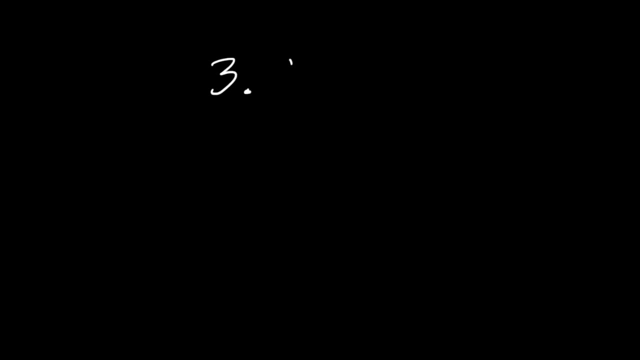 Now let's try another example. Let's multiply 3.9 by 5.6.. Feel free to try this one if you want to. So first let's multiply 9 times 6.. 9 times 6 is 54.. So we're going to write the 4 and then we're going to carry over the 5.. Next, let's multiply 3 times 6.. 3 times 6 is 18, and 18 plus 5 is 23.. 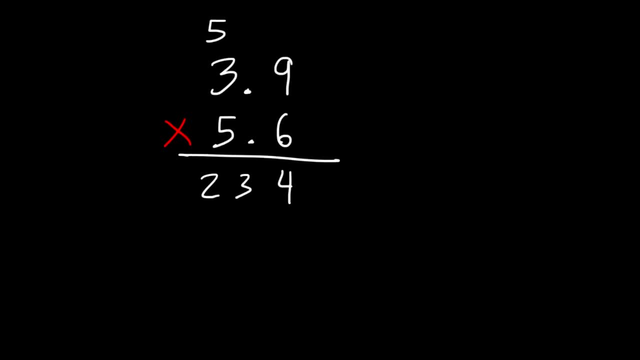 Now let's move on to the 5.. Let's multiply 5 and 9.. 5 times 9 is 45. So we need to write the 5.. But we need to add a 0 first, and then we'll write the 5 and carry over the 4.. 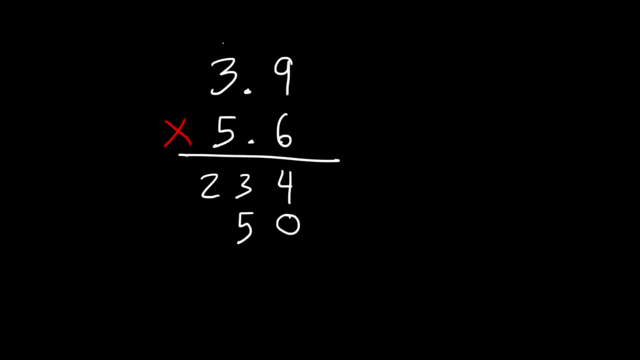 Next, let's multiply 5 times 3.. 5 times 3 is 15 plus 4.. That's 19.. Now what we need to do is add: 4 plus 0 is 4.. 3 plus 5 is 8.. 2 plus 9 is 11.. Carry over the 1.. 1 plus 1 is 2.. 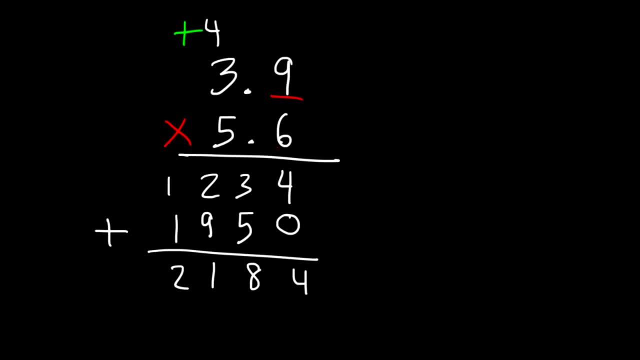 Now notice that we have two numbers to the right of a decimal point. So therefore in our answer we should have two numbers to the right of a decimal point. So the final answer is 21.84.. And that's it. Now let's multiply 12.4.. 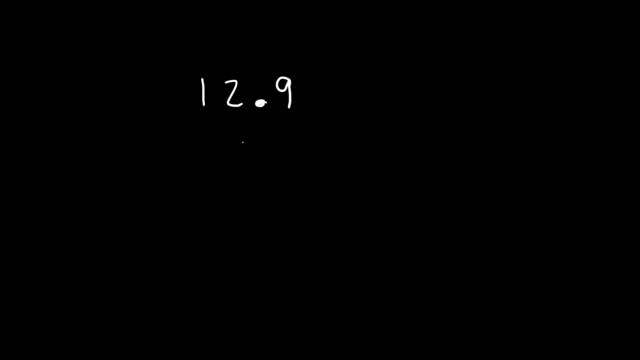 Now let's multiply 12.9 by 3.7.. Feel free to try this problem. So first let's multiply 9 times 7.. 9 times 7 is 63. So we're going to write the 3 and carry over the 6.. 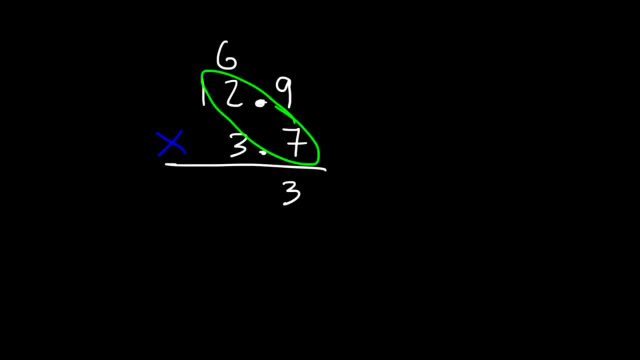 Next, let's multiply 2 times 7.. 2 times 7 is 14 plus 6.. That's going to be 20.. So we're going to write the 0 and carry over the 6. And carry over the 2.. 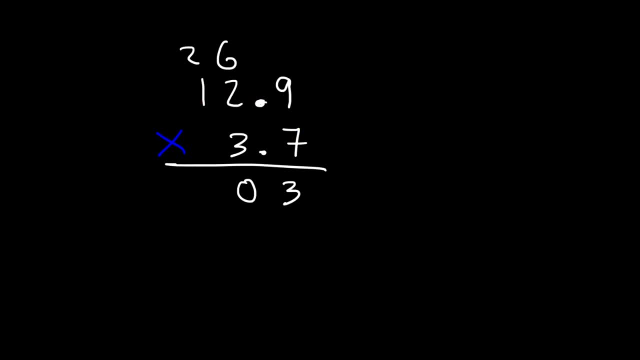 Next we have 1 times 7,, which is 7 plus 2. That's equal to 9.. Now let's add a 0. Let's get rid of these numbers. So now we're going to multiply 3 times 9.. 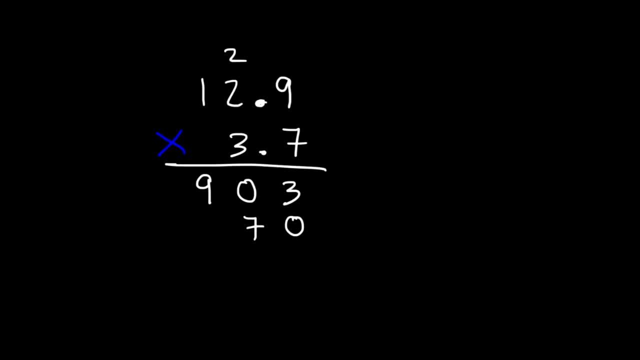 3 times 9 is 27.. Let's carry over the 2.. And then we'll multiply 2 times 3,, which is 6.. 6 plus 2,, that's 8.. And then finally 1 times 3,, which is just 3.. 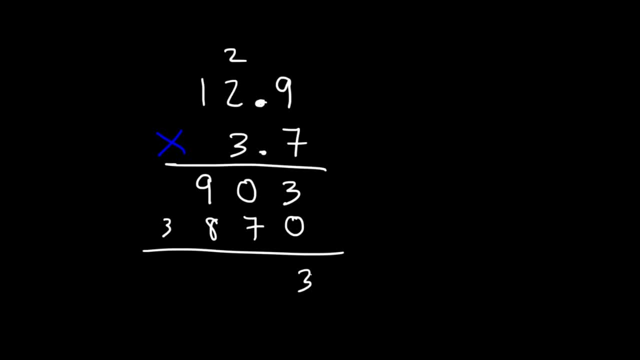 Now let's add the numbers: 3 plus 0 is 3.. 0 plus 7 is the same thing. 9 plus 8 is 17.. Carry over the 1.. 3 plus 1 is 4.. Now, how many numbers do we have? 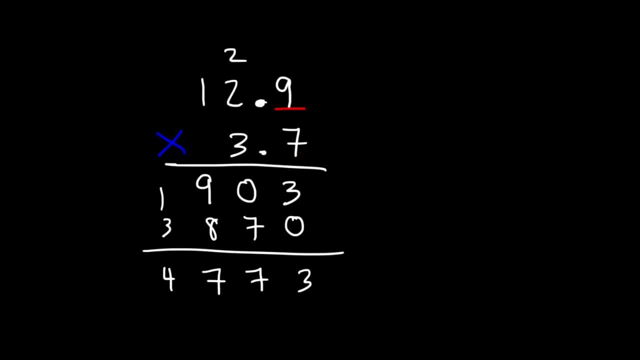 to the right of a decimal point. So here's one and here's another one. So we've got two numbers to the right of the decimal point. So we've got two numbers to the right of the decimal point. Our final answer should be the same. 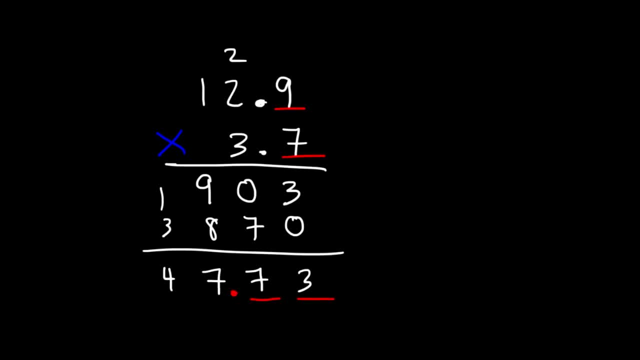 So these two numbers are going to be to the right of this decimal point. Therefore, the answer is 47.73.. Let's continue working on some more examples. Let's multiply 14.56 by 2.8.. So let's start with 8 times 6.. 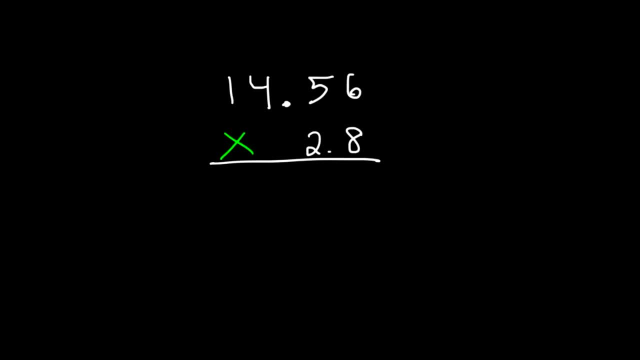 8 times 6 is 48.. Let's carry over the 4.. Next we have 8 times 5,, which is 40, plus 4. So that's 44. We're going to carry over the next 4.. 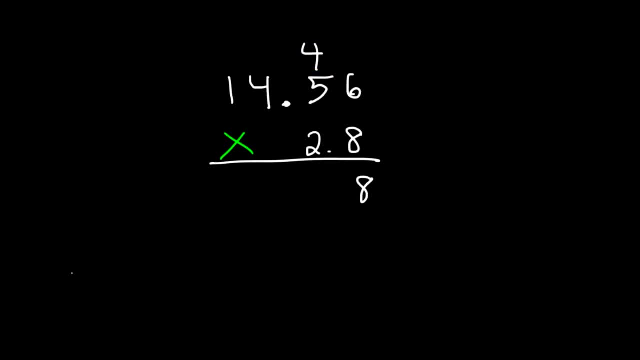 And then 8 times 4 is 32 plus 4.. That's 36.. So let's write: 8 times 4 is 32 plus 4.. That's 36.. We're going to write 6 and then carry over the 3.. 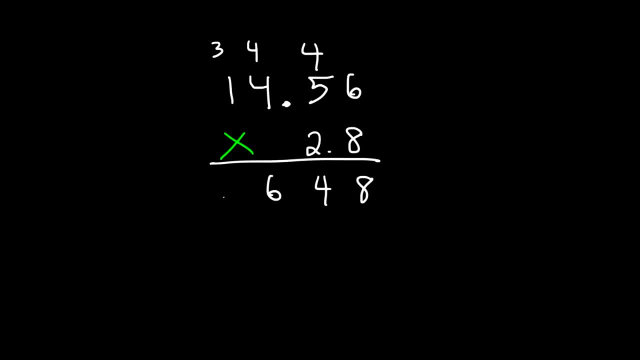 8 times 1 is 8 plus 3. That's 11.. So now let's get rid of these numbers. Let's add a 0 and then let's multiply 2 times 6.. 2 times 6 is 12.. 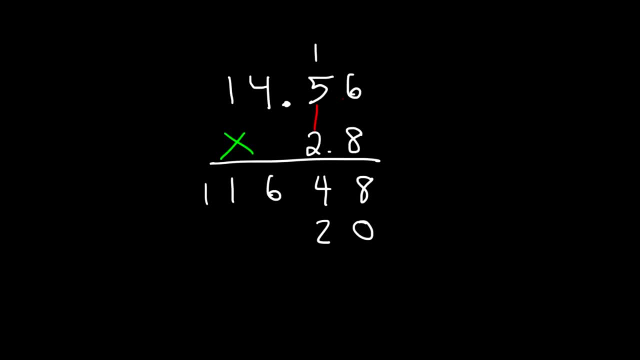 Let's carry over the 1.. And then 2 times 5 is 10 plus 1. That's 11.. So let's carry over the next one. 4 times 2 is 8 plus 1. That's 9.. 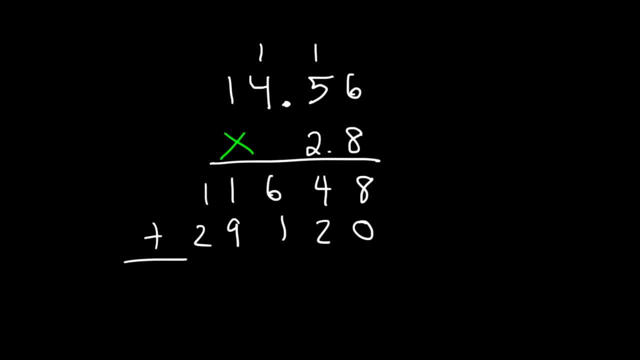 And then 1 times 2 is just 2.. So now we can add: So this is going to be 8.. 4 plus 2 is 6.. 6 plus 1 is 7.. 1 plus 9 is 10.. 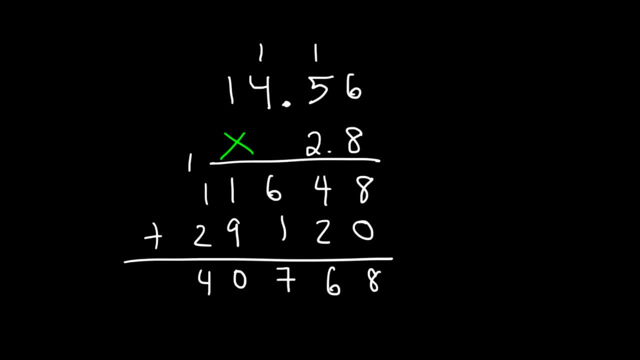 Carry over the 1.. 1 plus 1 is 2 plus 2 is 4.. Now where should we put the decimal? So, looking at the original problem, the first number has 2 digits to the right of a decimal point. 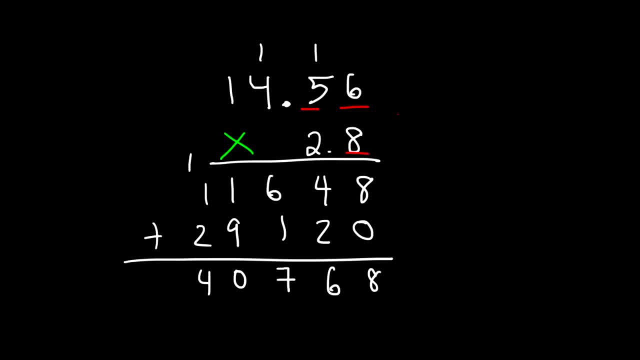 And the second number only has 1.. Therefore, our final answer should have a total of 3 numbers to the right of the decimal point. So therefore, the answer is 40.768.. 40.768.. Now let's move on to some harder examples. 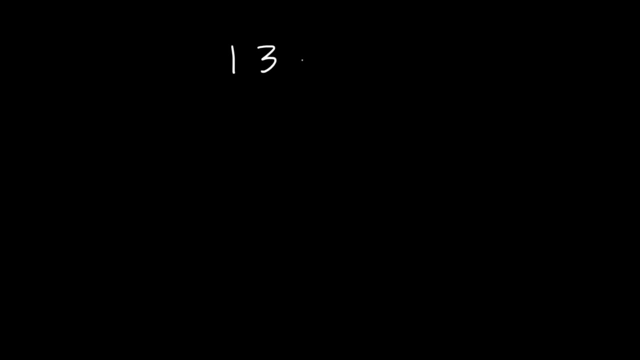 Now let's move on to some harder examples. Let's multiply 13.79, 13.79 by 5.46 by 5.46. So go ahead and try this problem. So go ahead and try this problem. Let's begin by multiplying. 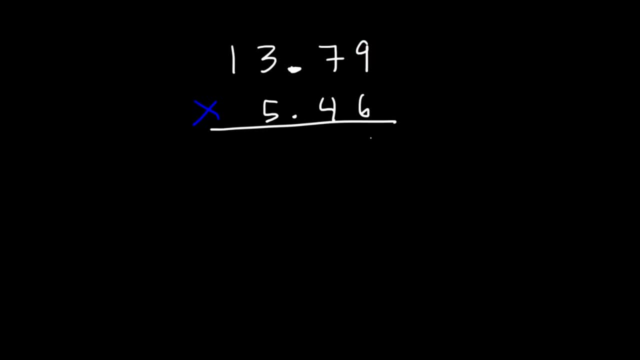 9 and 6.. 9 times 6 is 54.. Let's add the 5 on top. Next we have 7 times 6. Which is 42 plus 5.. So that's 47.. Let's carry over the 4.. 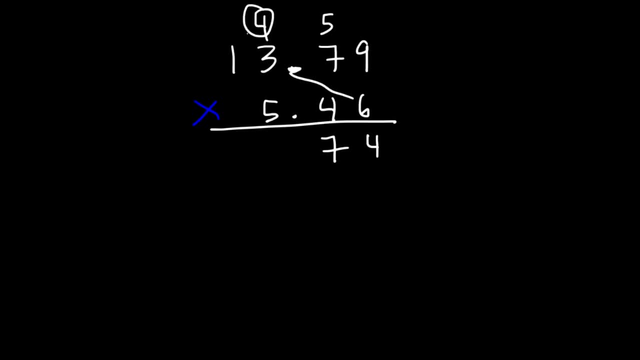 And next we have 6 times 3, which is 18 plus 4. So that's 22.. And now let's add the other 2 there. 6 times 1 is 6 plus 2. That's 8.. 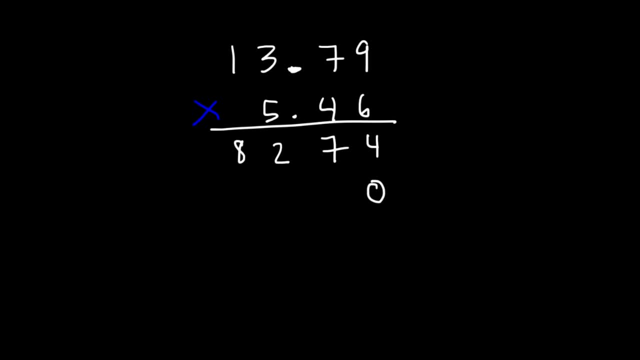 Now don't forget to add 0.. So we're done with 6.. Let's move on to 4.. 4 times 9,, that's 36.. So let's add a 3.. And then 4 times 7 is. 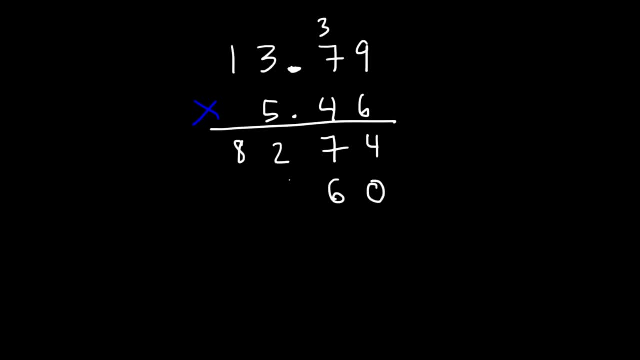 28 plus 3.. That's 31.. So let's carry over the other 3.. And then 3 times 4 is 12 plus 3.. That's 15.. So let's write 5 and carry over the 1.. 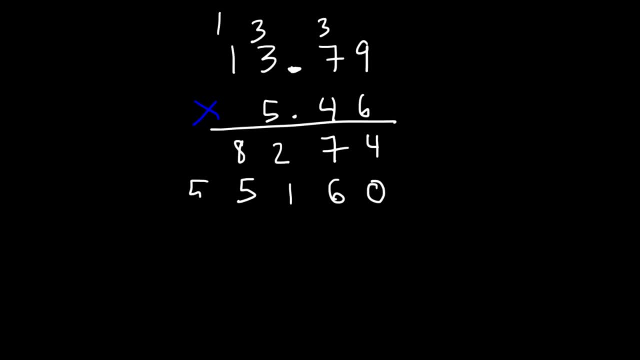 That's 4 plus 1. That's 5.. So now we're going to move on to 5.. Let's get rid of the numbers on top And let's add a 0. Actually, this time we're going to add 2 zeros. 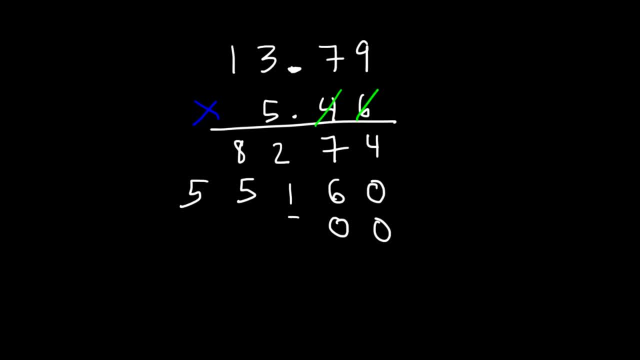 So now, 5 times 9, that's 45.. And then 5 times 7 is 35 plus 4.. That's 39. Carry over the 3.. 5 times 3 is 15 plus 3.. That's 18.. 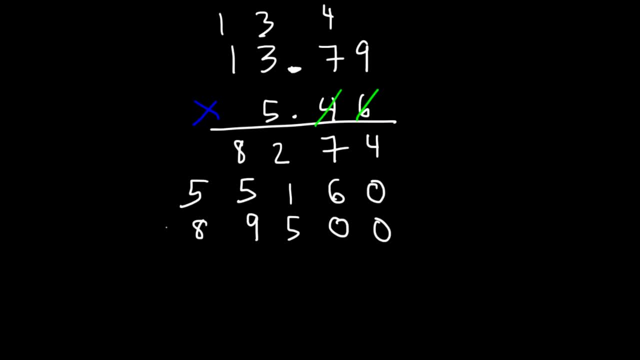 And then 5 times 1 is 5 plus 1.. That's 6.. So now let's add the numbers. So this is 4.. 7 plus 6 is 13.. And then 1,, 2 and 1. 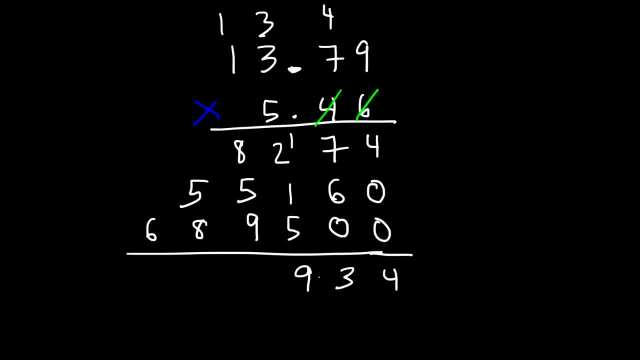 that's 4 plus 5 is 9.. 8 plus 5 is 13 plus 9, that's 22.. 8 and 2 is 10 plus 5, that's 15.. And 6 and 1 is 7.. 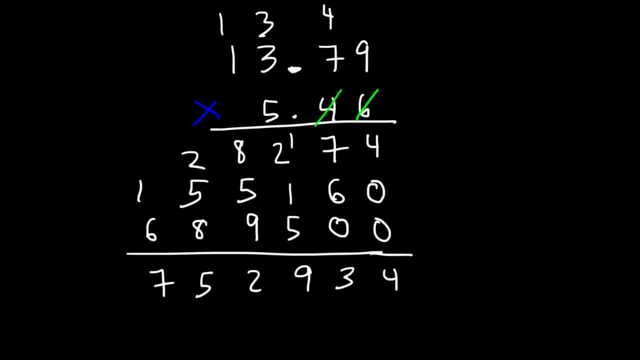 Now, where should we put the decimal? So, looking at the original numbers, the first number has 2 numbers to the right of the decimal point, And the second number also has 2 numbers. So therefore, our final answer should have a total of 4 digits.